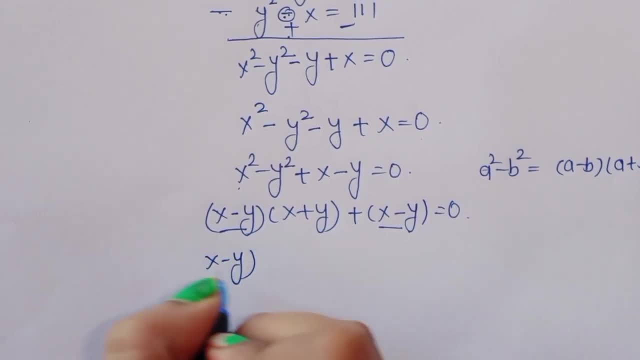 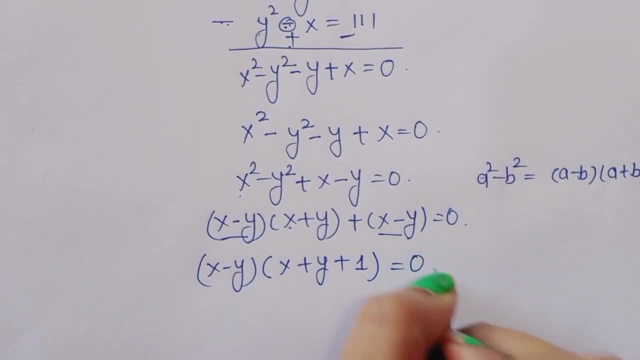 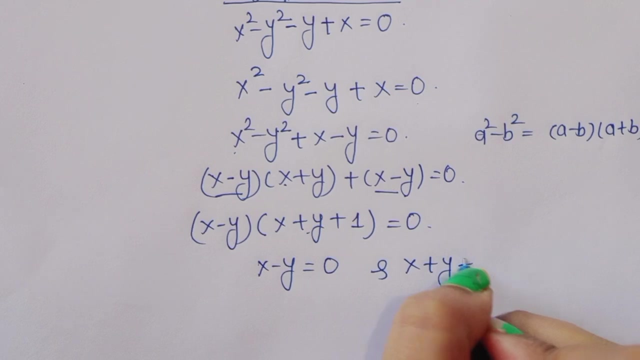 common. So we can take common here x minus y. Left term is: x plus y plus one is equal to zero. Now we can say: x minus y is equal to zero. And next one is: x plus y plus one is equal to zero. 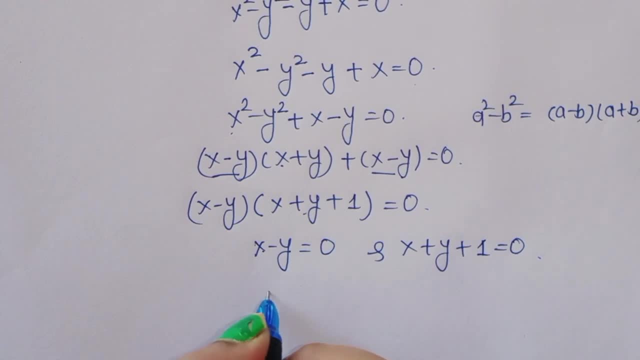 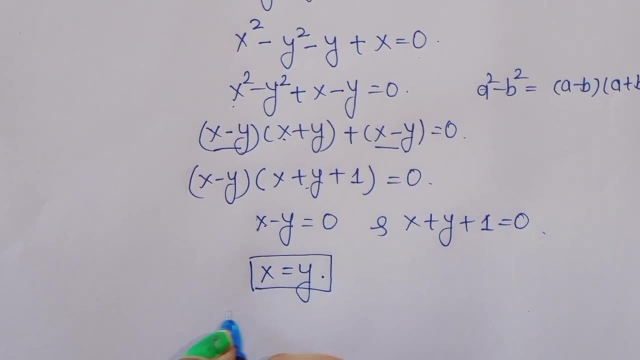 Now x minus y is equal to zero, So we can say x is equal to y, But x equal to y. This is not solution, Because condition is given x not equal to y. This is given condition there, So therefore this is rejected. 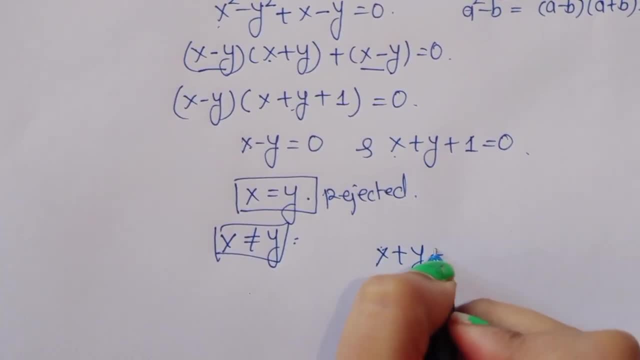 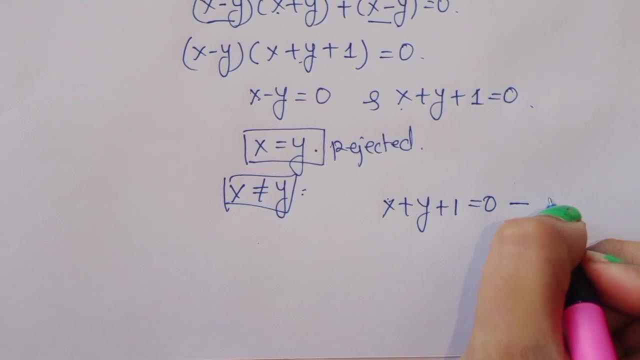 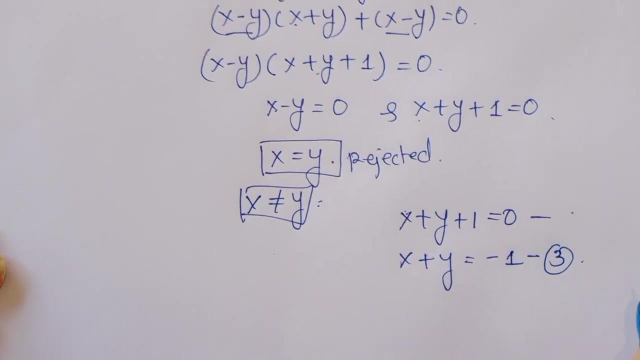 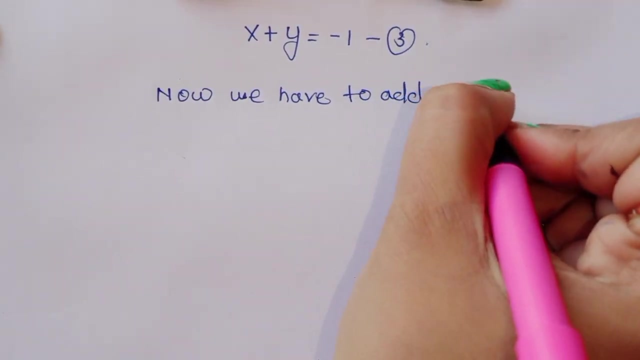 Next term is: x plus y plus one is equal to zero. Now we can write this: This is equation three. Or we can Right: x plus y is equal to minus one. This is equation three. To add Equation One and two, Then we will get. 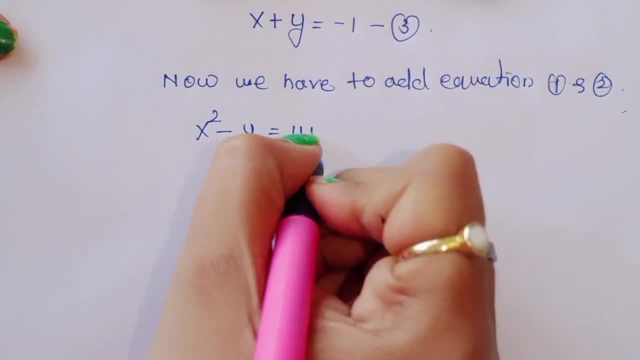 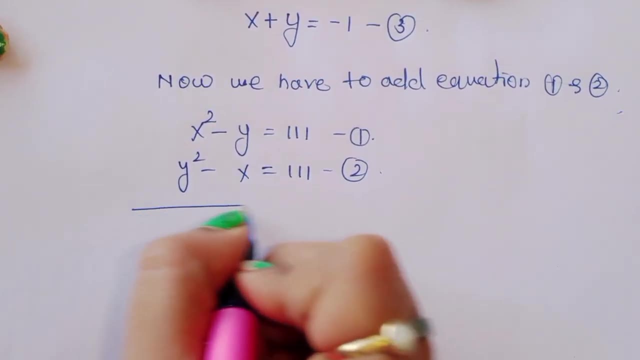 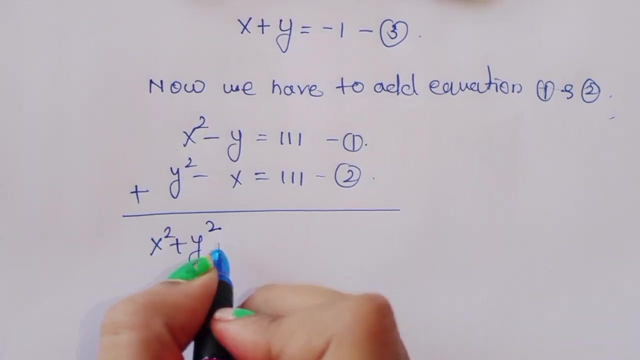 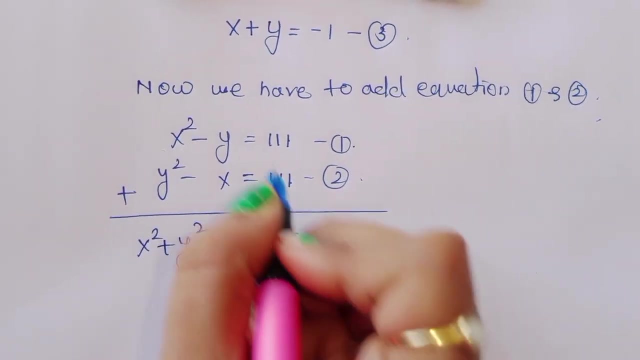 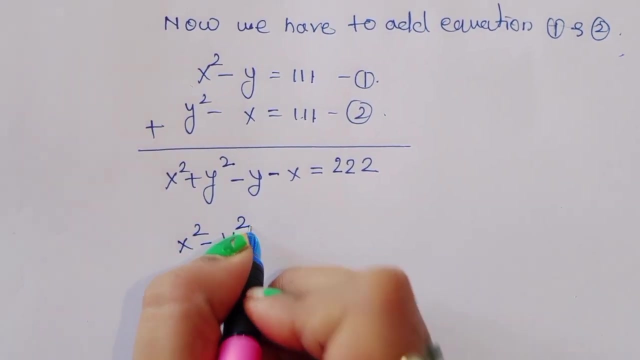 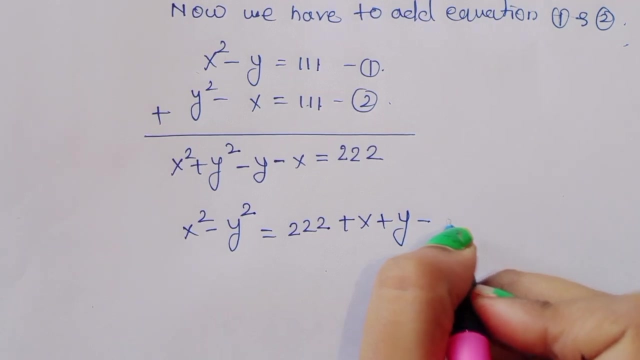 Equation one, that is x square minus y is equal to one hundred eleven. This is one, And y square minus x is equal to one hundred eleven. This is two. We have to add this one, Then we will get x square plus y square. x square plus y square minus x, minus y minus x is equal to one plus one, two, one plus one, two, one plus one, two. so we can write this: x square plus y square equal to two hundred twenty two plus x plus y. now this is equation four. 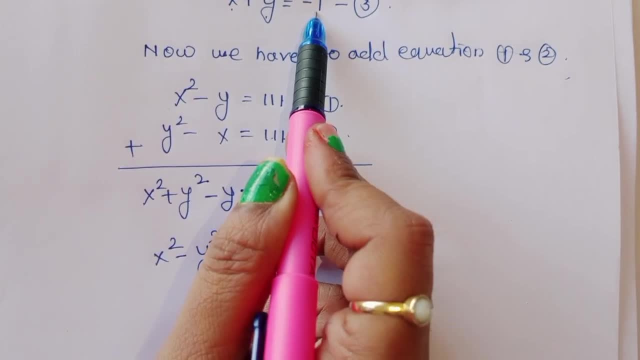 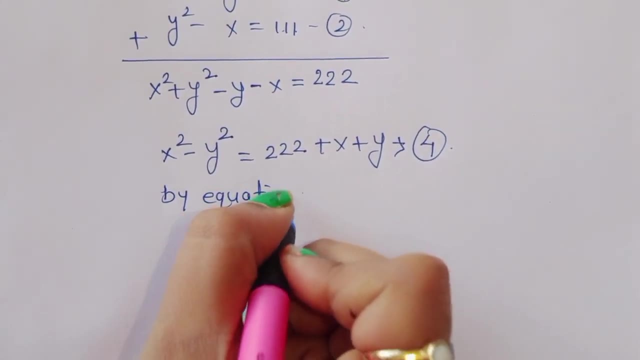 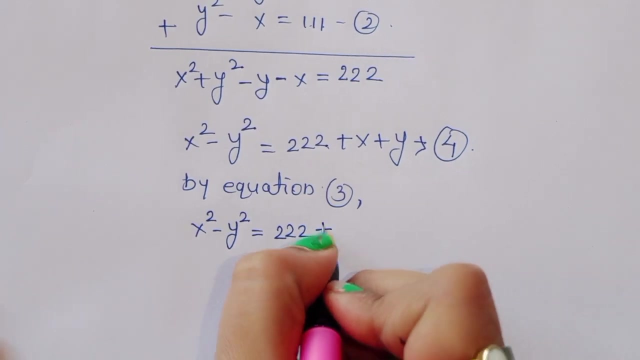 But we know the value of x plus y. x plus y is equal to minus one. This is given in equation three. So by equation three Minus y, square is equal to two. twenty two Plus X plus y. x plus y is equal to. 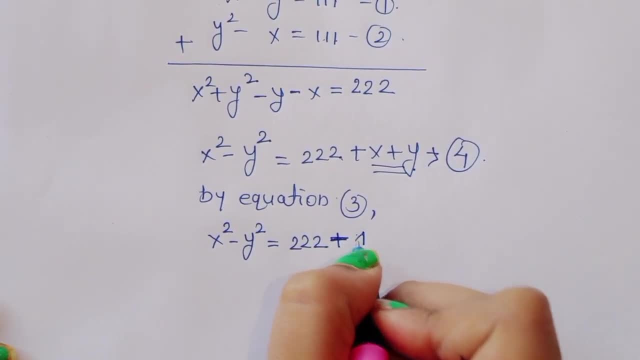 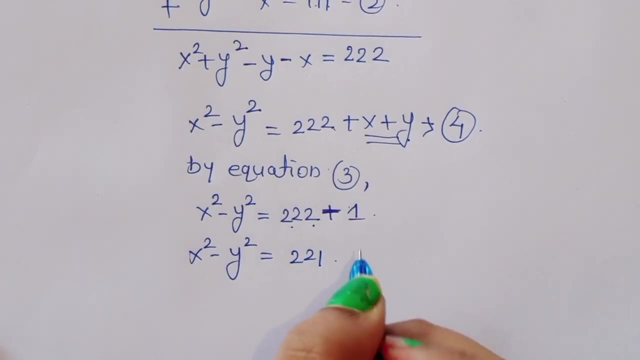 Minus one, so we can write this here Minus one. So x square minus y square is equal to Two twenty two Minus one, that is two twenty one. This is equation five. We got here value of x square minus y square. 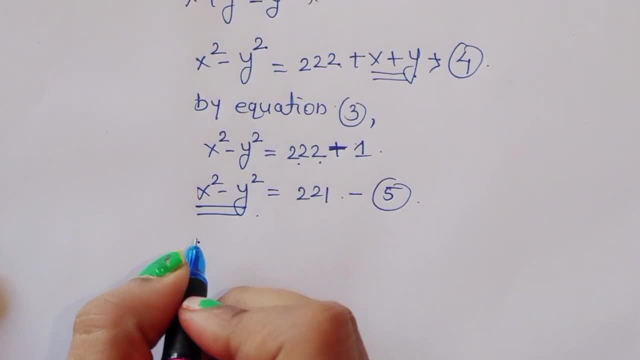 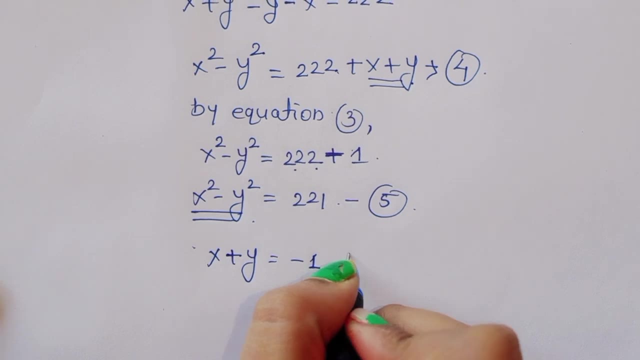 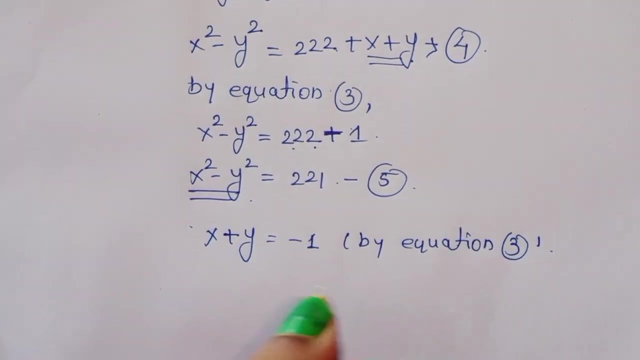 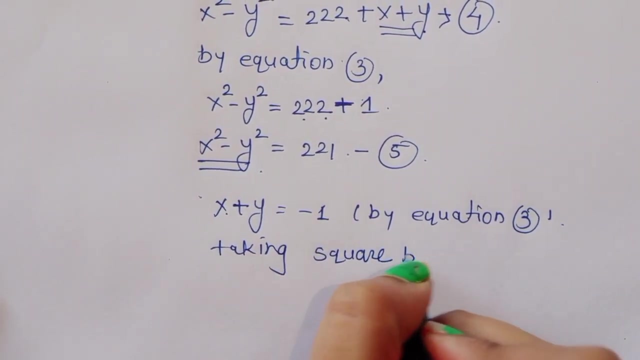 Now taking square both side. We can take equation three: X plus y is equal to minus one. This is equation three. Or we can write by equation Three: This is we got value Then: x plus y. taking square. now Taking square. 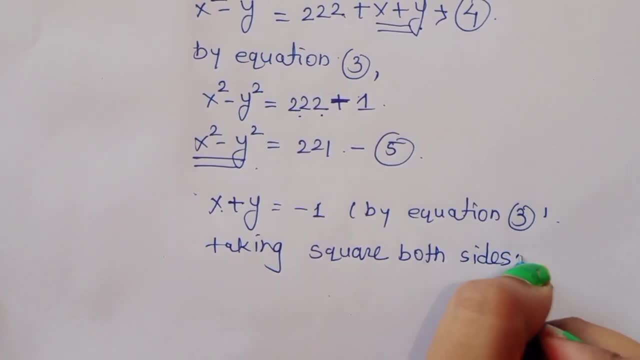 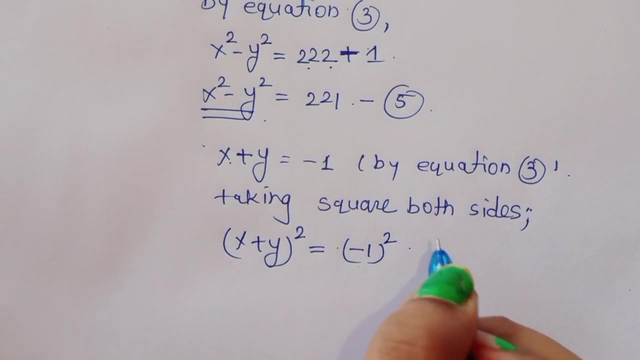 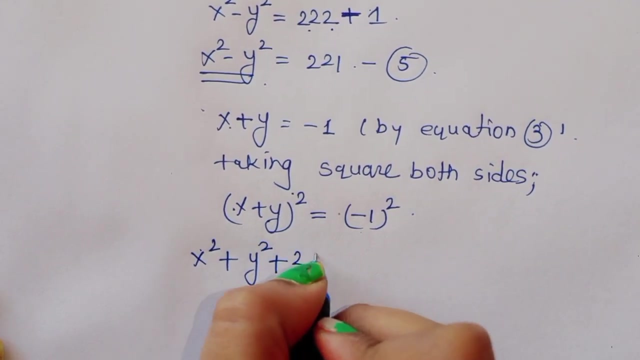 Both side, Both sides, we will get here: X plus y- whole square is equal to minus one square. Now x plus y- whole square. We can write this: x square plus y square plus two, x, y is equal to minus one, That is, plus one square of minus one. 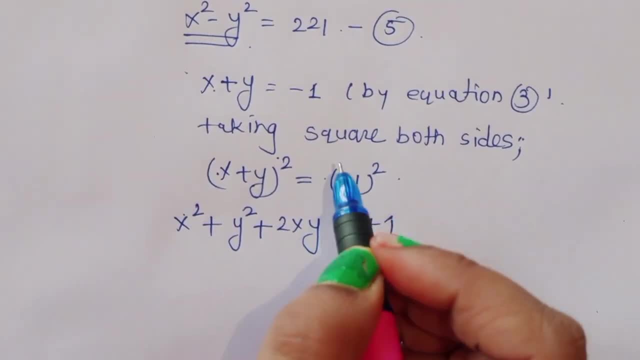 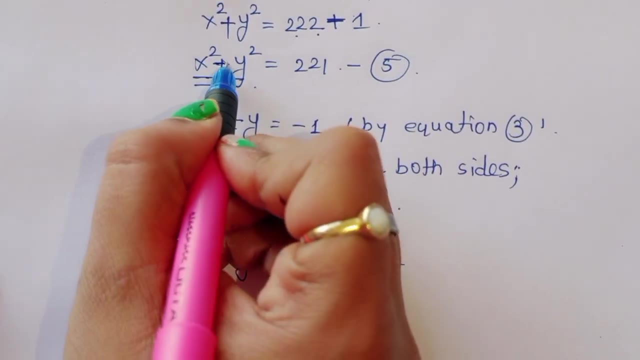 That is plus one. Now you can see here: This is the value of x square plus y square, x square minus y square, y square, x square plus. this is plus x square plus y square. x square plus y square is equal to two twenty one. 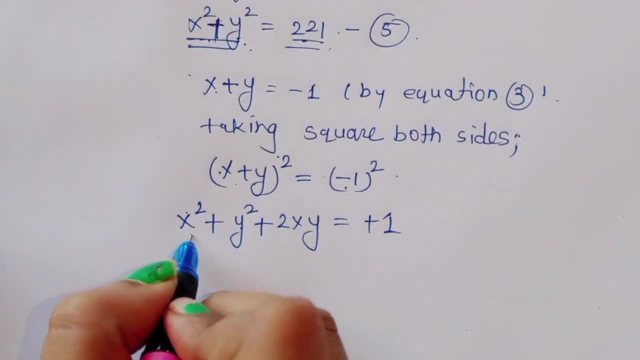 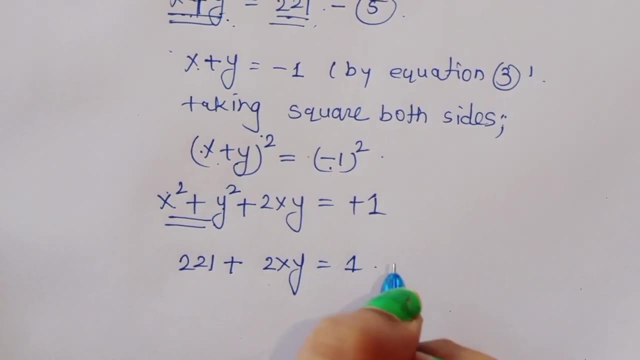 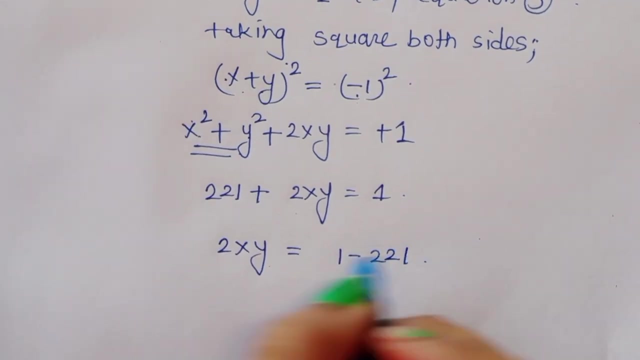 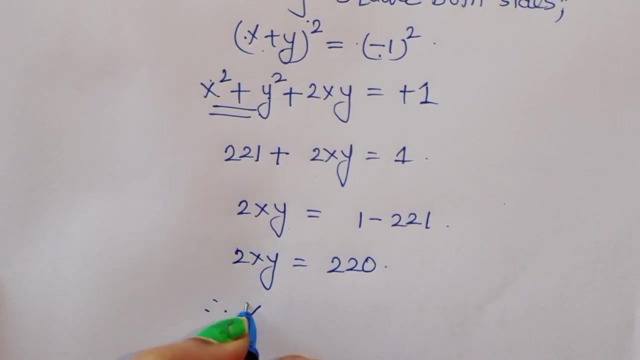 Now value of x square plus y square two twenty one. We have to substitute here: Now two twenty one plus two x- y is equal to one. So we can write this: two x- y is equal to one minus two twenty One, 1.. And 2xy is equal to 220.. Therefore we can say value of xy is equal to 220 divided. 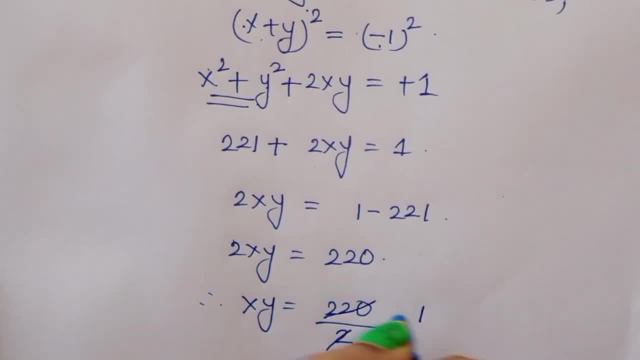 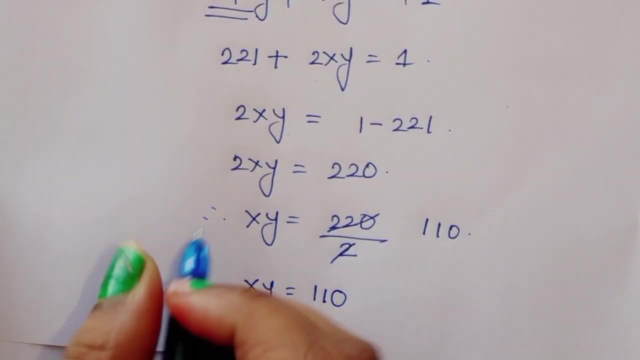 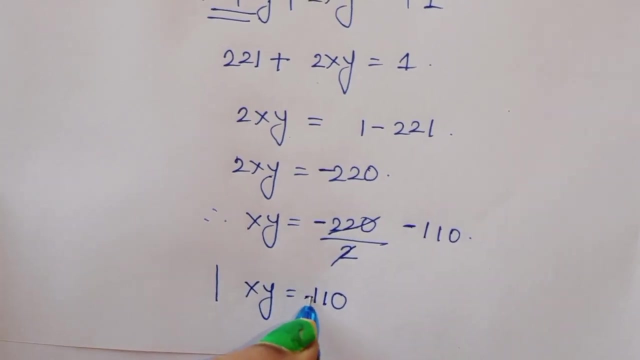 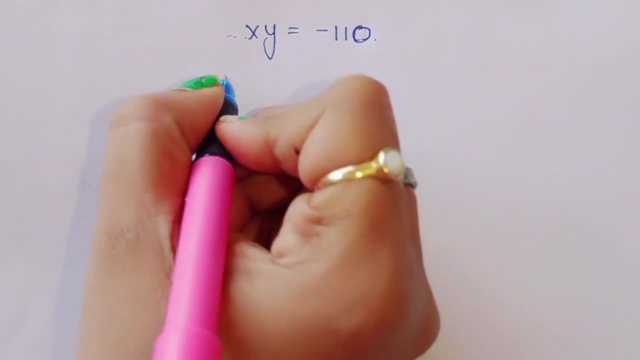 by 2.. 2 x 2,. 2 x 2, 110.. Value of xy is equal to 110.. This is minus 220.. So minus 110.. Value of xy is equal to minus 110.. xy is equal to minus 110. Therefore, we can say y is equal. 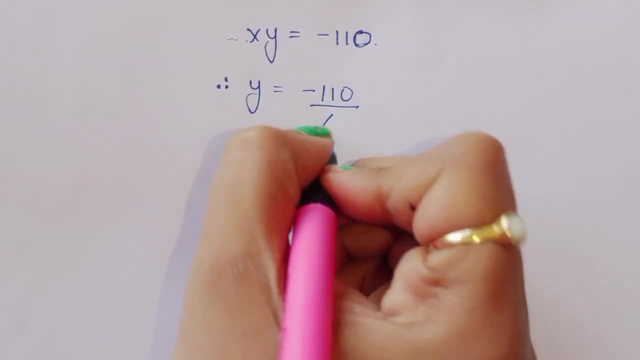 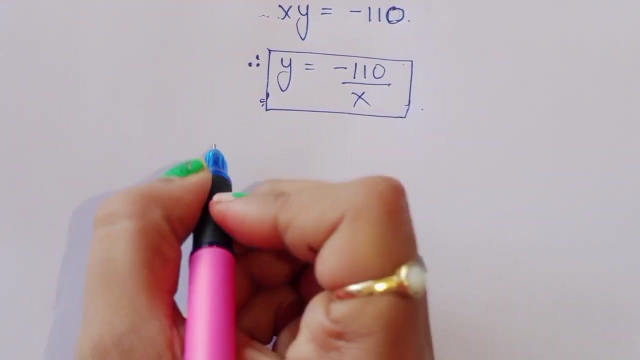 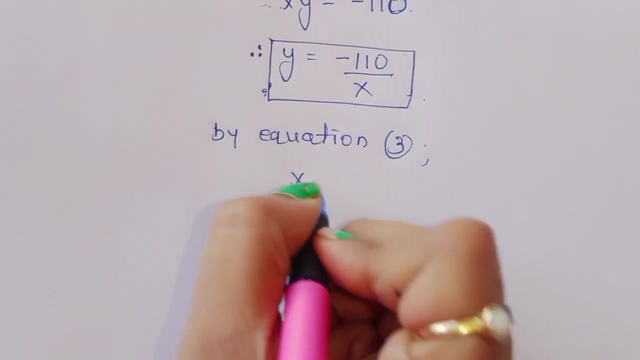 to minus 110 divided by x. This is the value of y. Now we have to find out the value of x. Then we can say by using equation 3.. By equation 3, x plus y is equal to minus 1.. 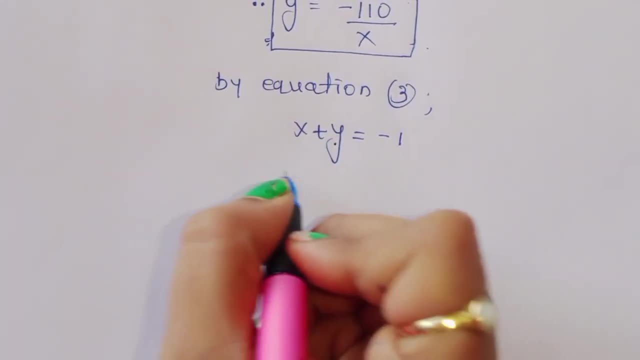 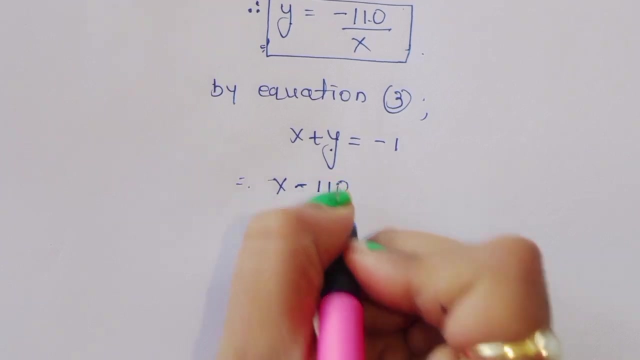 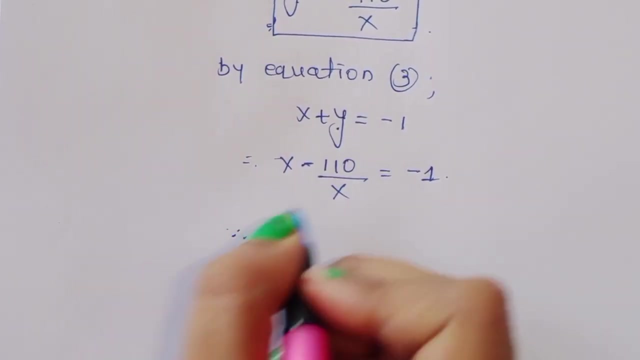 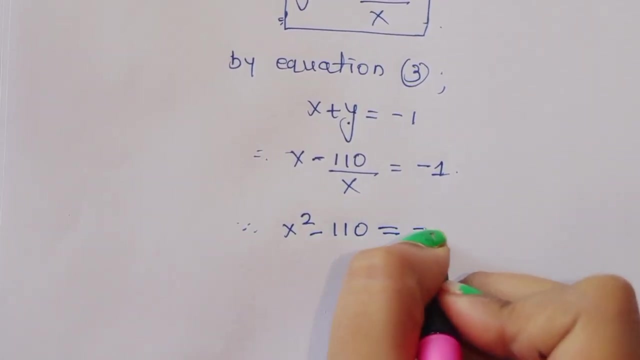 Now we can say: can substitute value of y here. Then therefore, x plus y, that is minus 110, divided by x is equal to minus 1.. Now here we can say: when we are simplify this one, then we will get: x square minus 110 is equal to minus x. or we can write this: x square plus x minus 110. 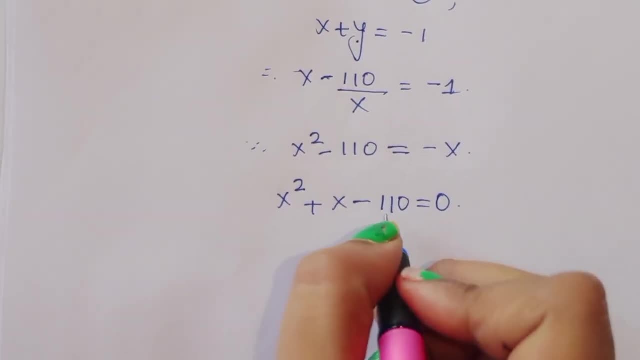 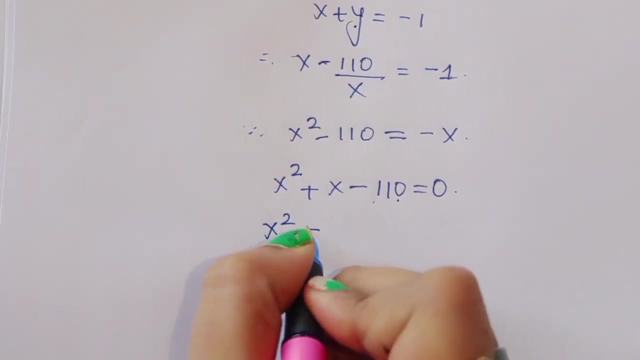 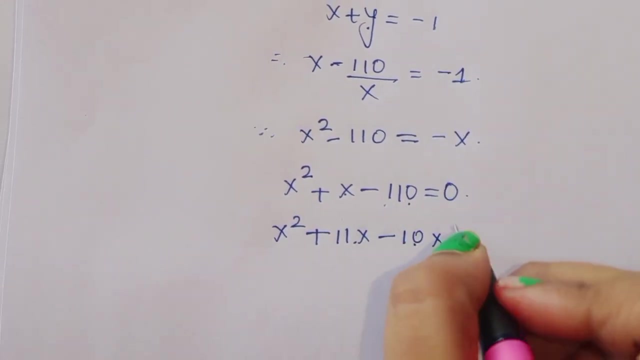 is equal to 0.. Now 11 tanja, that is 110.. So we can write this: x square plus 11x minus 10x. 11x minus 10x, that is x. So we can write this: x square plus 11x minus 10x. 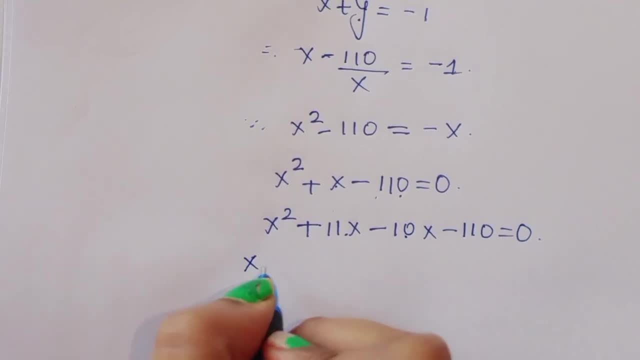 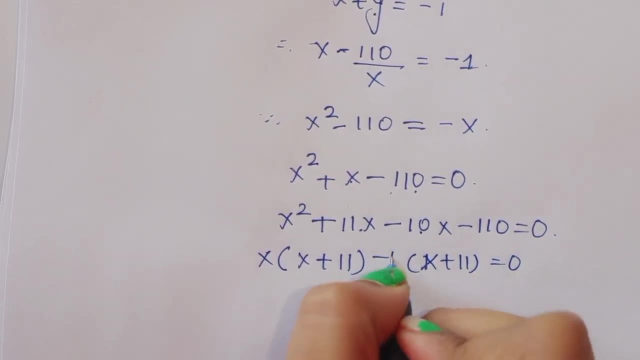 So we can write this: x square plus 11x minus 10x. So we can write this: x square plus 11x minus 10x minus 110 is equal to 0.. Now taking common x, here x plus 11,. x plus 11 to 0, here minus 10,. 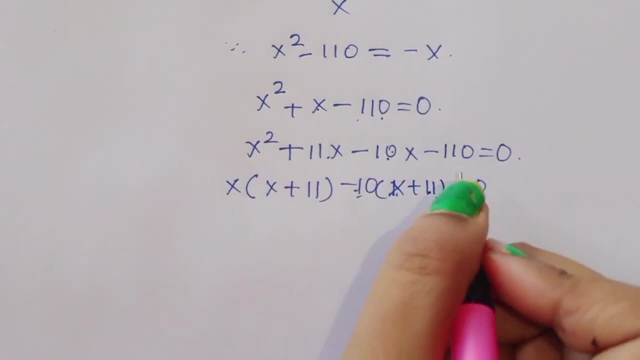 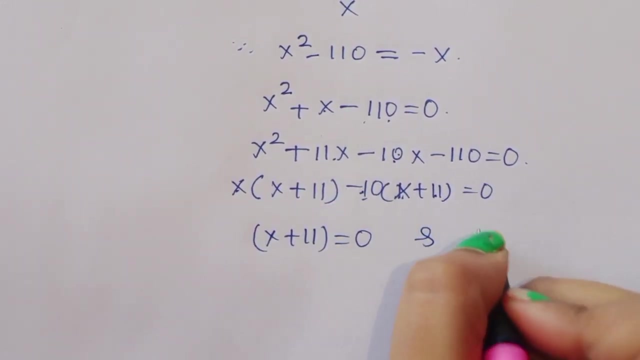 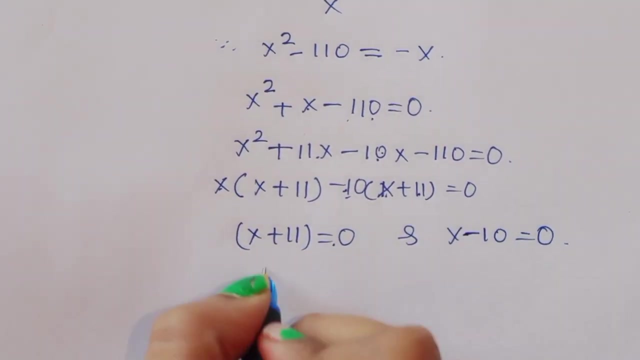 minus 10x minus 10 into 11,, that is 110.. So x plus 10 equal to 0, and next one is x minus 10, x plus 11 equal to 0 and x minus 10 equal to 0.. Now x is equal to. we can say here: x is equal. 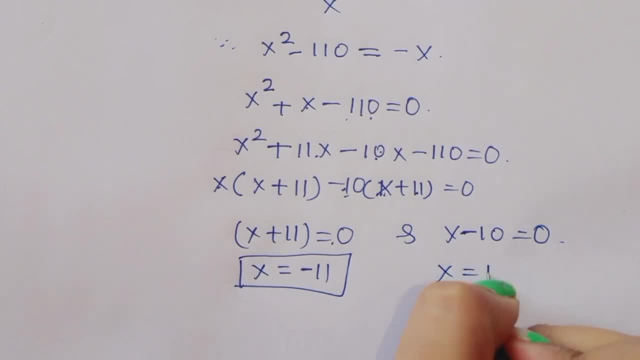 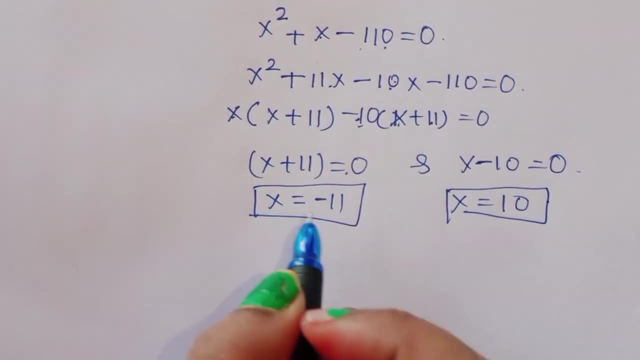 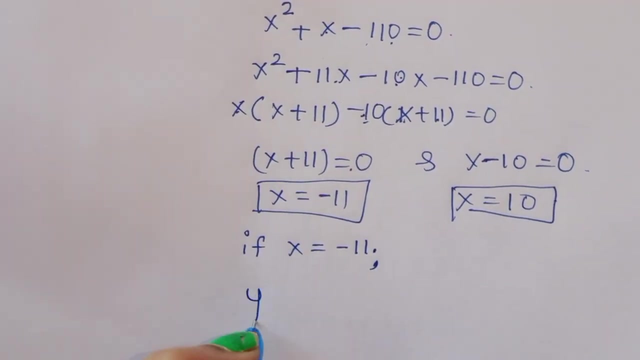 to minus 11, and here x is equal to 10.. Now, if x is equal to, we have to find out the value of now y. If x equal to minus 11, at that time y equal to. we can say y equal to. 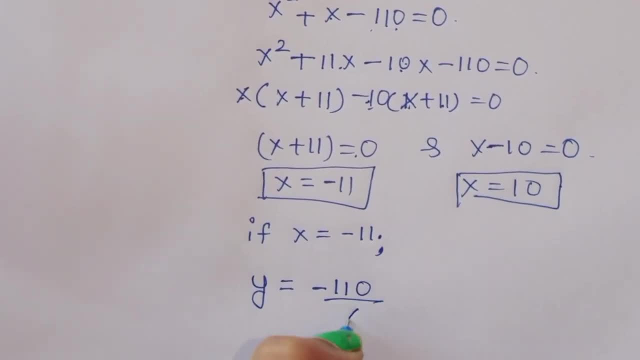 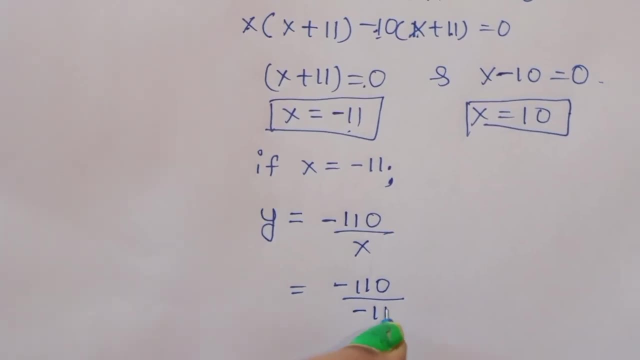 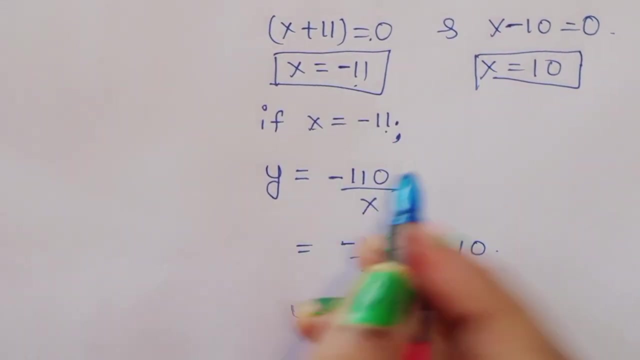 minus 100.. So y equal to minus 110 divided by x. Therefore, y equal to minus 110 divided by x, that is minus 11.. So 11, this is 10.. Therefore, in that time value of when x is equal to minus 11,. 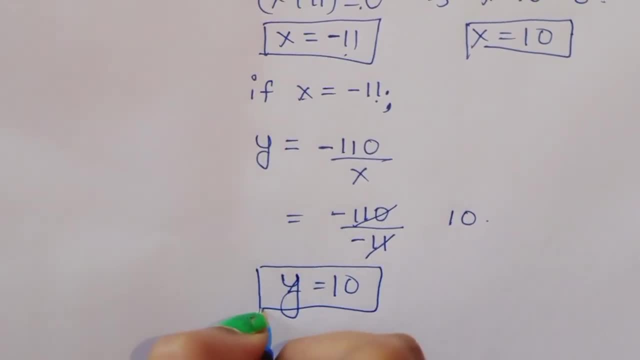 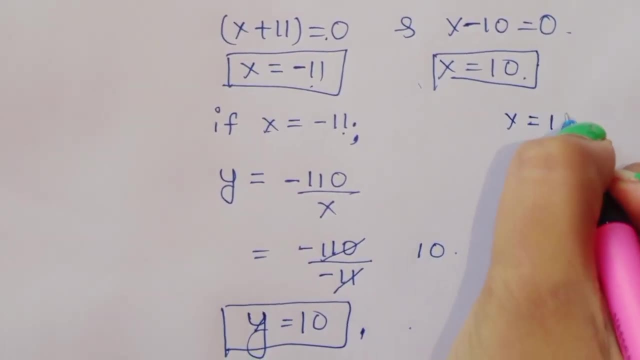 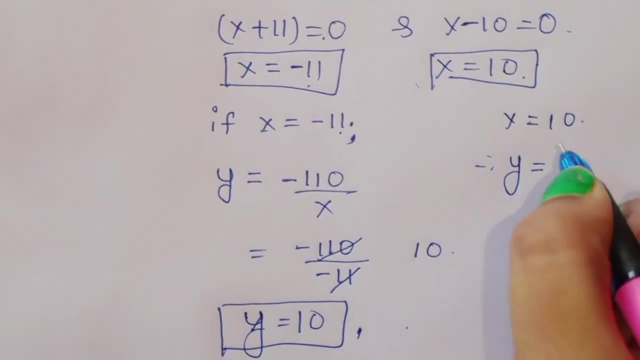 at that time value of y is equal to 10.. And in next term, when x is equal to 10, at that time we can say: when x is equal to 10.. Therefore, y equal to value of x. that is, value of y that is 100, minus 110 divided by 10.. Therefore, y is equal to.